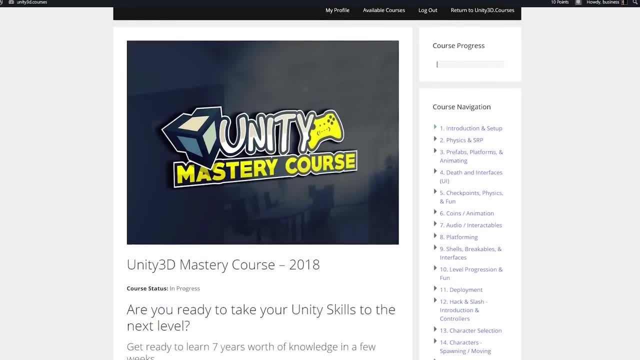 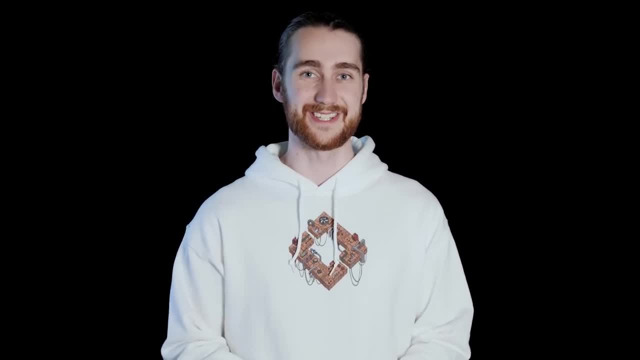 If you sign up for his course now, will also get access to his Game Dev Mastery course, which will teach you how to build a variety of game types. So simply click the link in the description to get a headstart with your coding skills. So arm yourself with a keyboard and a cup of coffee. 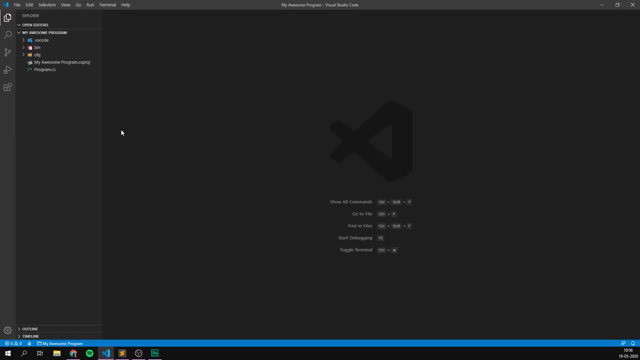 and let's get CODING. So we're here in VS Code and, as you can see, if we open the programcs file, there's some default code inside. Now this might look really scary to you, but don't worry, worry, You don't need to understand everything that's going on. In fact, we can ignore everything. 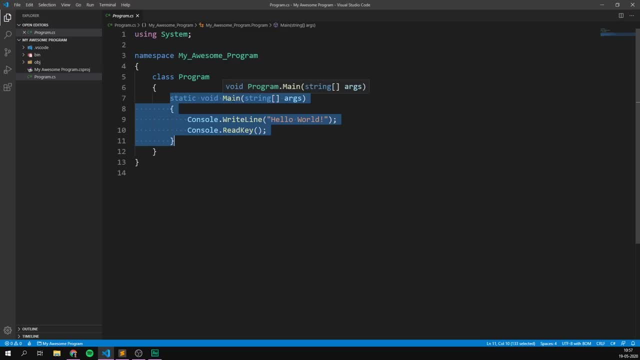 except this: This is a method called main and it's the place where we're going to put our code inside. We call this the entry method because it's called when our program starts. In other words, the stuff that we put inside of these two curly brackets is going to run when we open our program. 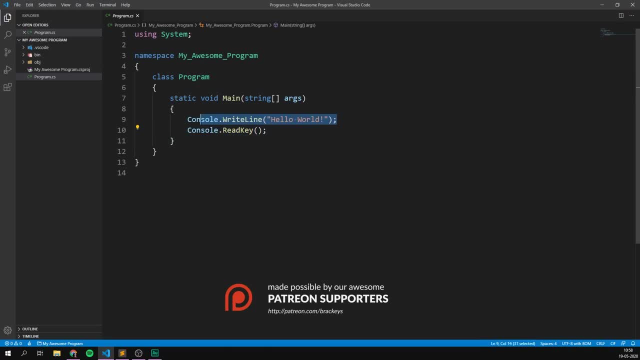 Right now we just have two lines inside of this method. The first one prints out the words hello world in our console. The second one we added when setting everything up in the last video. This line waits for the user to press a button. This is just here to prevent our program. 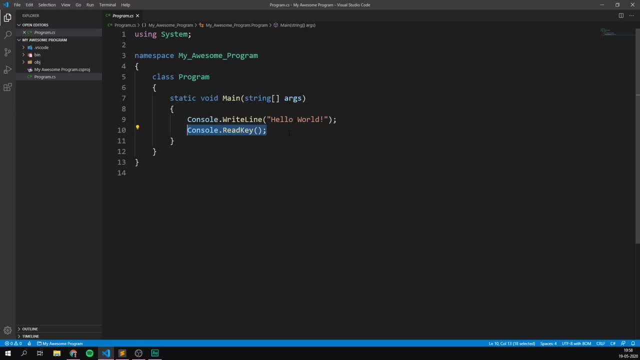 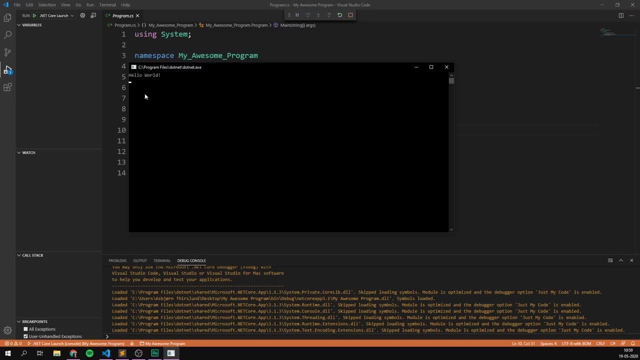 from ending and the window from closing before we press a key first. And indeed, if we go ahead and run this program now, by going run, start debugging, we can see that it just opens up a window that says hello world, And when we press a key it closes. So let's try and write some code here. 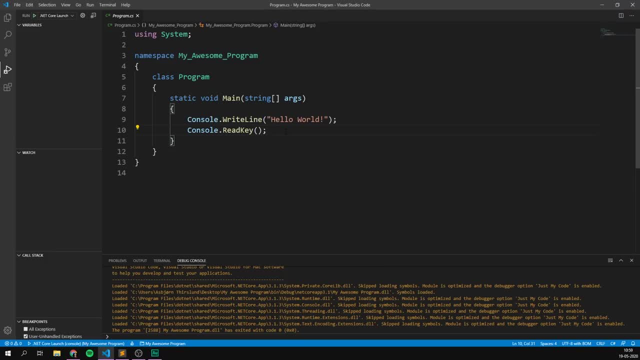 to make it more exciting. First of all, we can actually change the appearance of our program. So let's try and write some code here to make it more exciting. We do this by going to the top of our code here and making a few lines Again, remember. 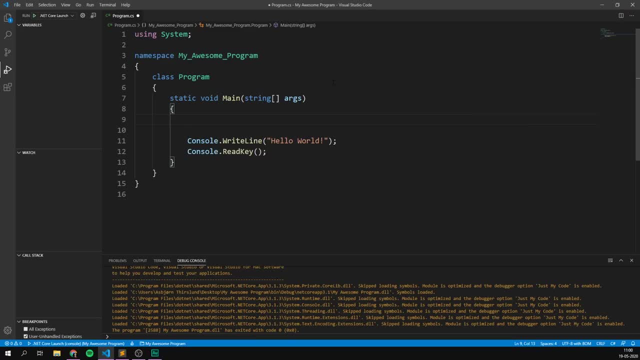 this needs to be inside of these two curly brackets, And here we're going to write console, because we want to access the console and change something about it. Console in this case. here is what we call a class. You can think of a class like a container with a bunch of things. 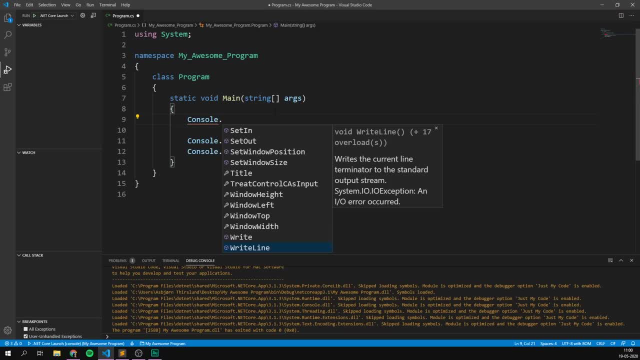 inside. If we write a dot here, we can access all the things inside the console class. As you can see, there are a bunch of different things here that we can use, And most of these has one of two icons: either a wrench or a box. The wrench means that it's a 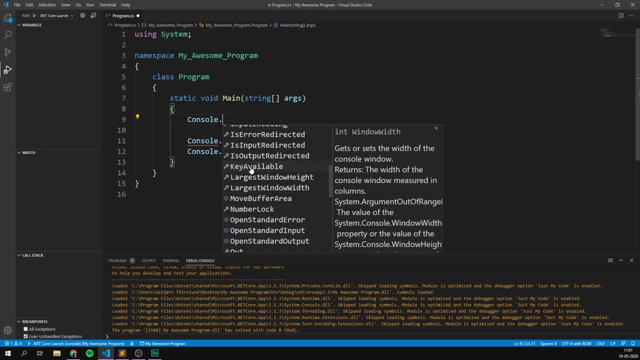 variable or a property. These are things that we can change about our console, such as color, title or size. The box, however, means that it's a method or a function. These are commands that we can call in order to have a console do different things, such as write out a line of text or wait. 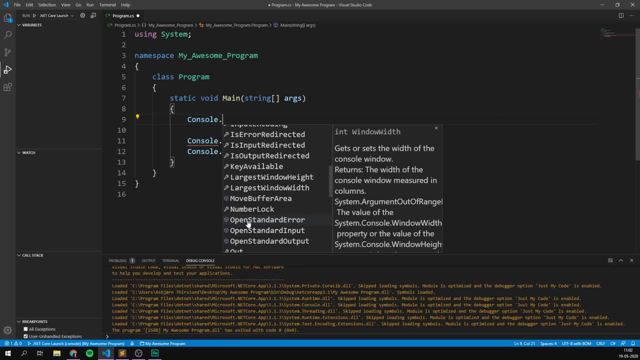 for the user to type something in. So if, for example, we want to change the window title of our console, we can do that by going to the console, And if we want to change the window title of our console, we should look for a property that does this. So we could either scroll up and 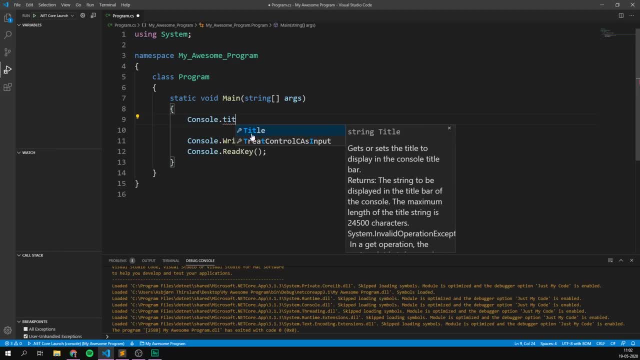 down here or we could begin typing: I'm going to type in title here And indeed there's a property here called title, So I'm going to hit enter in order to auto-complete that, And we can now change this title by simply setting it equal to whatever we want. So I'm going to make an equal sign here. 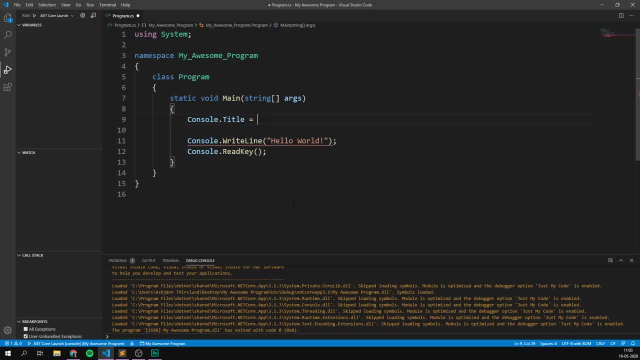 And whenever we're dealing with text, we want to make sure to put it inside of two quotation marks. So I'm going to call my console Skynet, So those of you who've watched Terminator- And after this line is done, we want to go ahead and insert a semicolon. 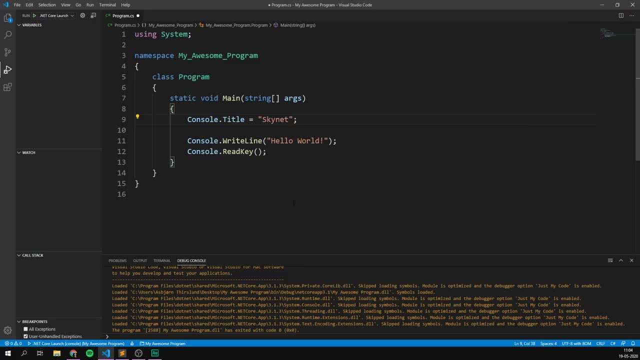 In general, if you're writing code that tells our program to do something on this line, we end it with a semicolon. Things like remembering to put a semicolon, knowing when to put in quotation marks, and all of this stuff is what we refer to as syntax. 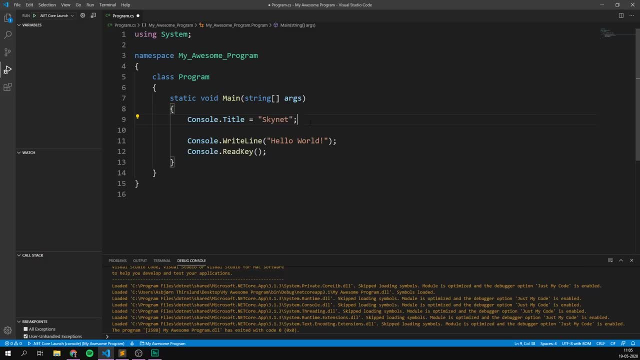 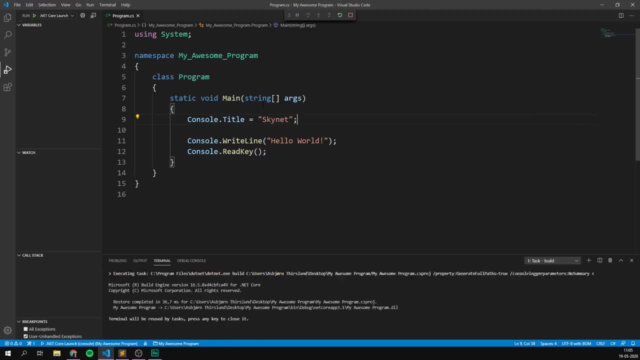 In the beginning it might feel awkward and a bit scary, but don't worry, you get used to the syntax very quickly. So now, if we go ahead and run our program here- whether you go up here or just press F5, we can see that indeed. 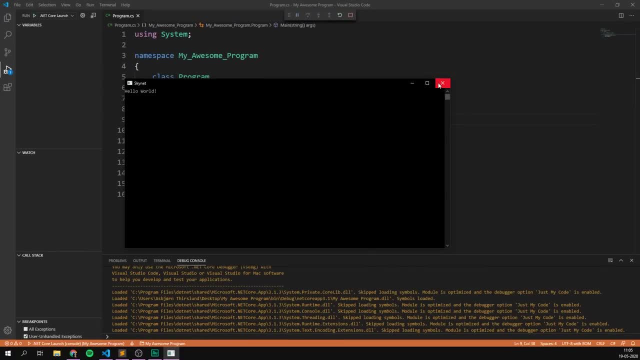 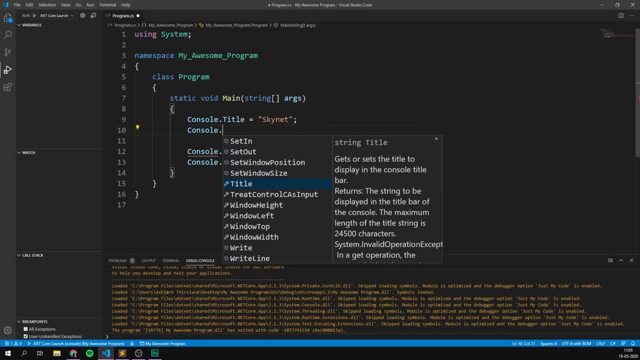 we've now changed the window title to Skynet Awesome, And we can actually also change the color of our text. This is just as easy: We just go console And this time we look for a property modifying color. So I'm going to search for color here And, as you can see, 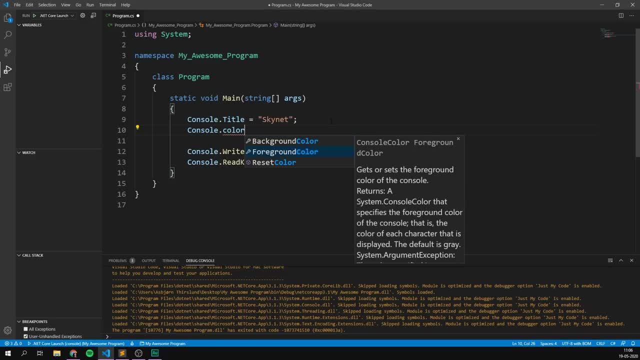 there's both a background and a foreground color. I want to modify the text, so I'm going to choose foreground color here, And let's go ahead and set that equal to And, in order to see the different colors that we can choose between. 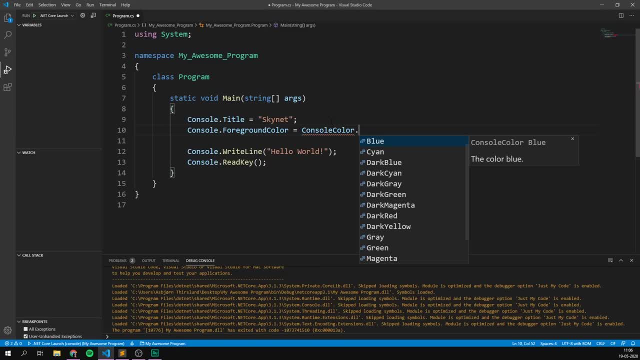 we're going to go ahead and hit enter, And we're going to go ahead and hit enter And in order to see the different colors that we can choose between, we are going to write console color dot. And here we get a bunch of options. 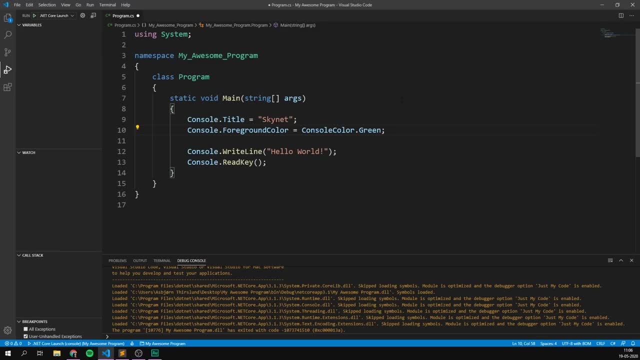 So I'm going to set mine to a programmer's green and simply end that line with a semicolon. And indeed, if we now run our program, we can see that the text is green. Awesome, And we can even change the size of the window itself. 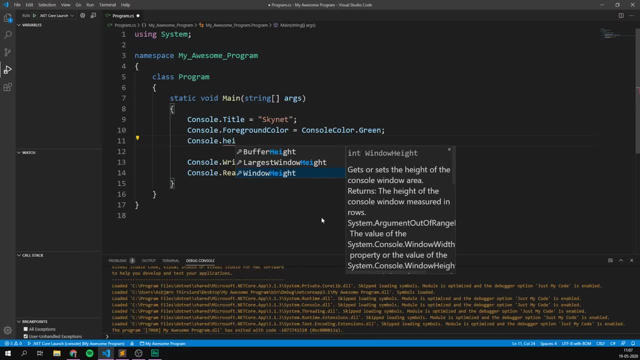 Let's do this by going console and let's go ahead and change the window height, And here we can just set this equal to some number, And the number is going to represent how many lines tall our window is going to be. So I'm going to set this to 40 or 40 lines tall. 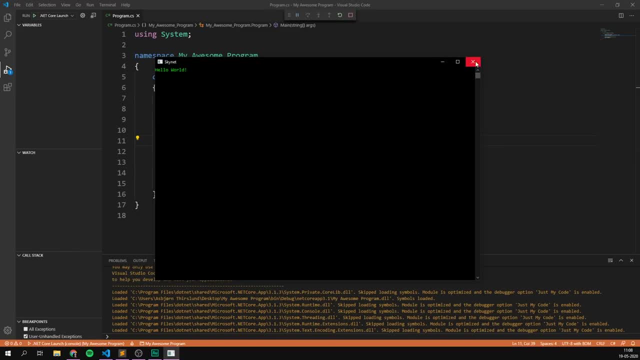 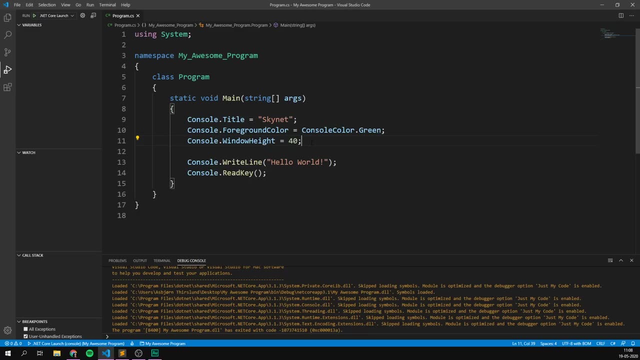 And, as you can see, our window is now much taller. Awesome, So that's how you can modify properties in order to change the appearance of your console. Now let's go ahead and write something more exciting that actually makes our console do things. 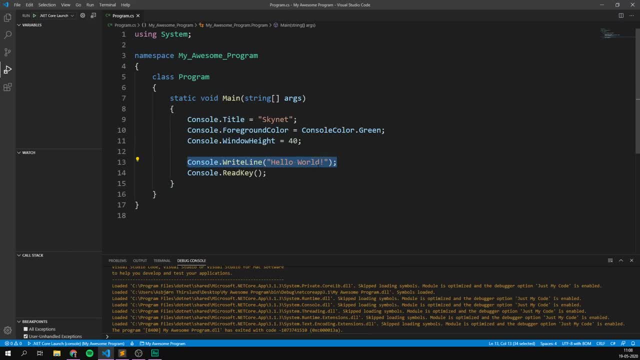 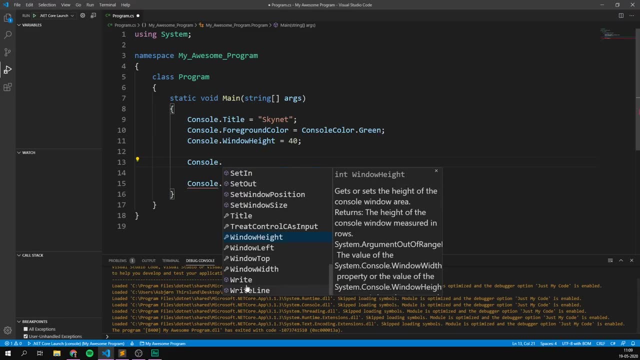 So I'm going to get rid of this line right here that says hello world, And instead I'm going to write my own. So I'm going to write console dot, And here we want to look for a method. So one of the boxes here 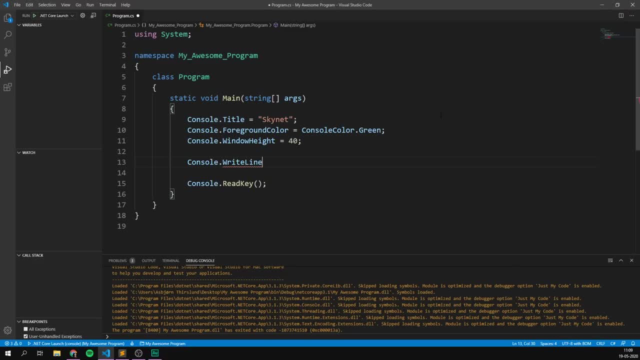 I'm going to again put in a right line here, And whenever we are calling a method, we want to put in an open parenthesis, close parenthesis followed by a semi-colon. So I'm going to put in an open parenthesis here. 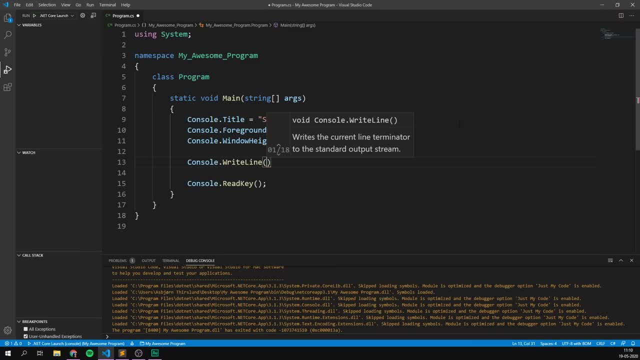 As you can see it, auto completes the other one, And before we put in our semi-colon, this method would like to know what it should write. This is called an argument. Arguments are values that we give to the method to use. 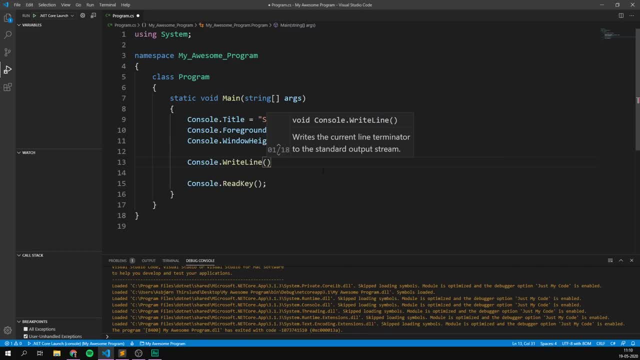 Some methods don't take any arguments, while others can take many different ones. As you can see, we have a method called argument. As you can see here, this method actually takes 18 different arguments. We can give it a whole number, a decimal number. 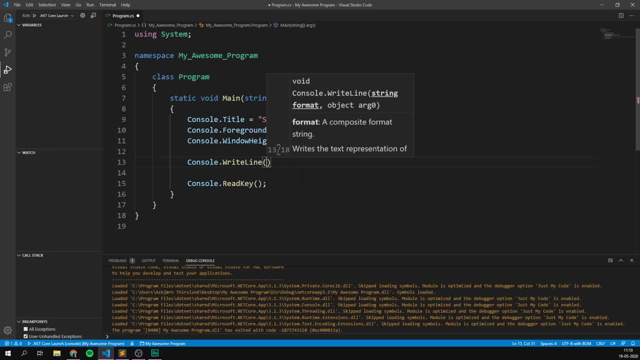 some text and so on. So there's a bunch of options for us here. In our case, we want to give it some text. So, again, we're dealing with text here. So we remember to put this inside of quotation marks and I'm going to write: hello, what's your name? 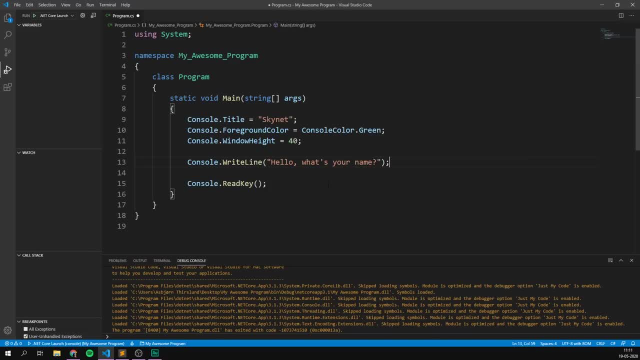 And again, let's finish the line with a semi-colon. So now we're writing hello, what's your name in the console? Then we can have the user type in their name. To do this, we use another method. Let's create some new lines here. 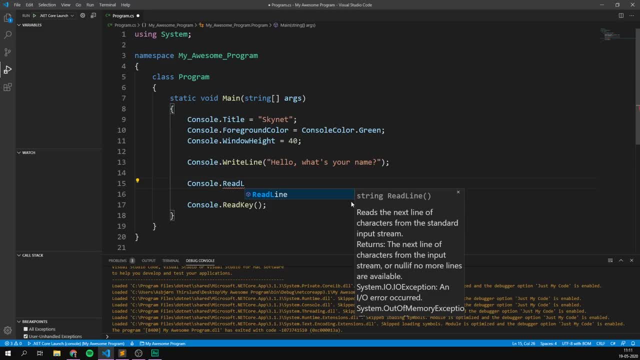 And for this we write consolereadLine. So just like we can have the console write a line on its own, we can also read a line from the user, And again, this is a method. So we're going to open and close two parentheses. 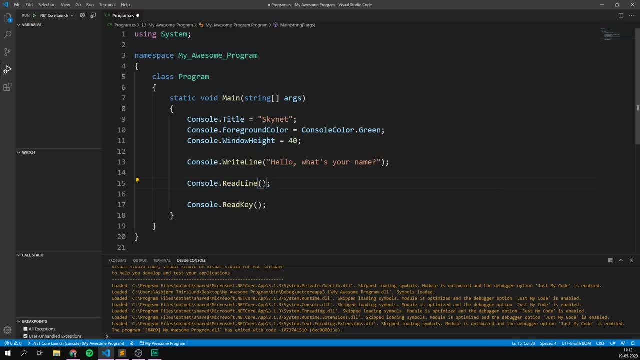 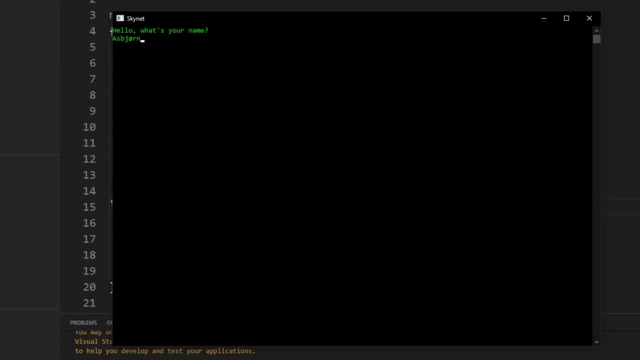 and put in a semi-colon. As you can see, this method doesn't take in any arguments, And if we now run this program, we can see that it asks for our name. I'm going to go ahead and put my name here and not much more happens. 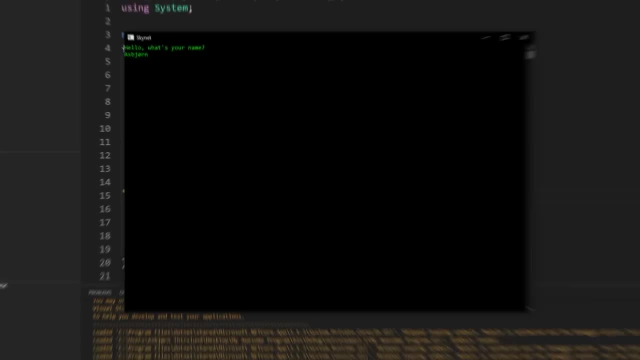 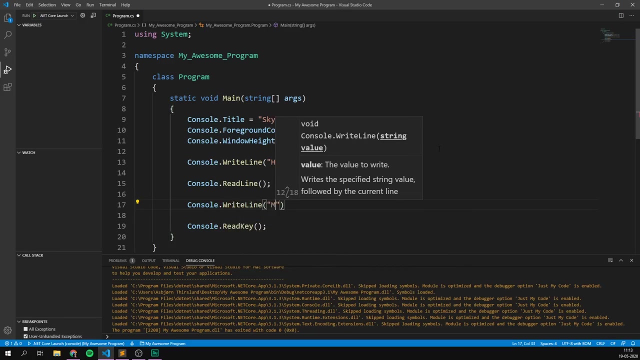 but so far we are kind of starting to get a conversation going. So let's simply add some more code to make it more interesting, Let's add another consolereadLine and I'm going to have it say: my name is RX 9000. 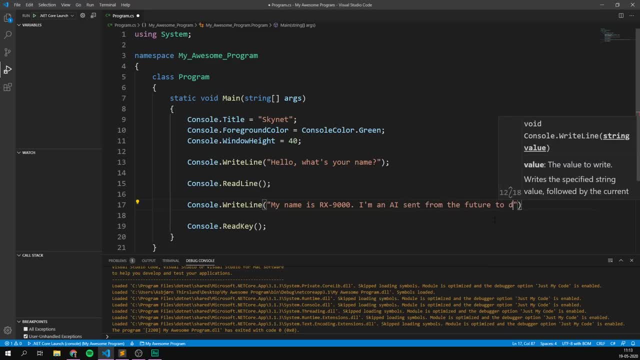 I'm an AI sent from the future to destroy mankind and end that with a semi-colon, And then we can have it write another line. So consolereadLine again what is your favorite Color? And there are actually two ways to create a new line. 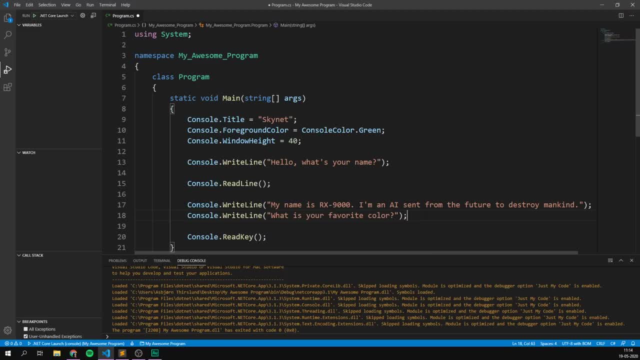 One is the one that we're using here. We simply split it up into two consolereadLines, And that is, of course, going to write two lines. However, we don't actually need to call the function twice. Instead, we can go inside of the text itself. 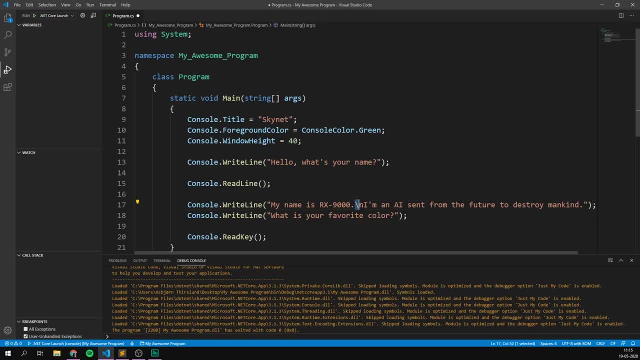 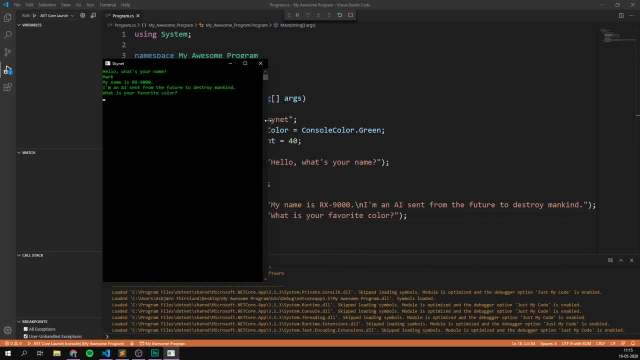 and put in a backslash end. This also creates a new line. So right now, if we run this- and I'm just going to type in Mark here- we can see that it says my name is RX 9000, just like we wrote it here. 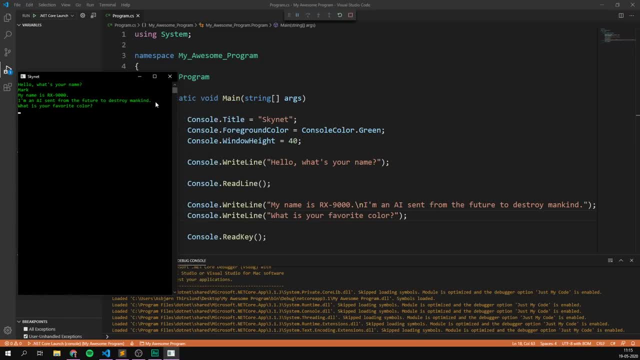 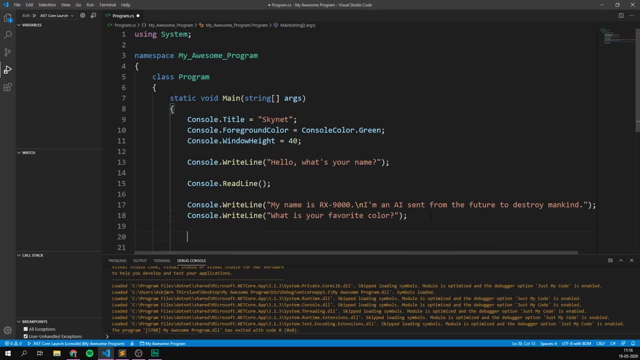 Then it creates a new line- I'm an AI sent from the future to destroy mankind. And then it creates a new line, again with a different method. What is your favorite color? So let's go ahead and add a readLine here so that we can input our favorite color consolereadLine. 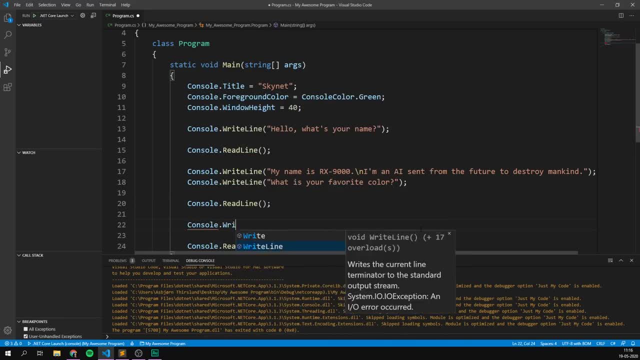 And then we can have the program answer with consolereadLine. cool Mine is destruction And indeed, if we run this now, we get to type in our name. And indeed, if we run this now, we get to type in our name. 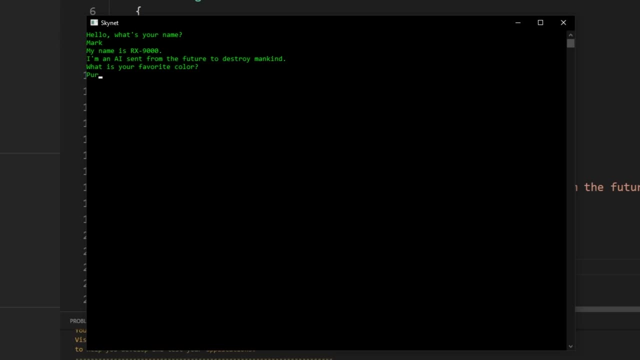 And indeed, if we run this now, we get to type in our name. It asks us for our favorite color. I'm going to type in purple here And it says: cool, mine is destruction. I think this AI means business. 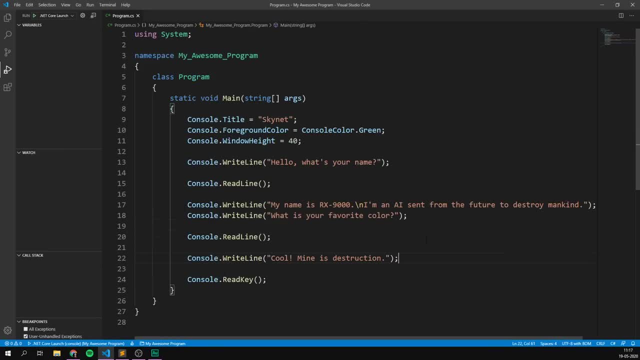 And that's our first custom program. Now I know that this can be a lot to take in, So sometimes it can be handy if you can write comments in your code to help you remember what is going on. This is actually really simple. If we go to the top here, we can maybe add a comment. 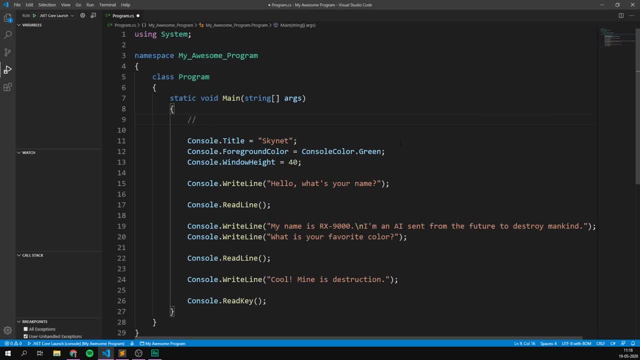 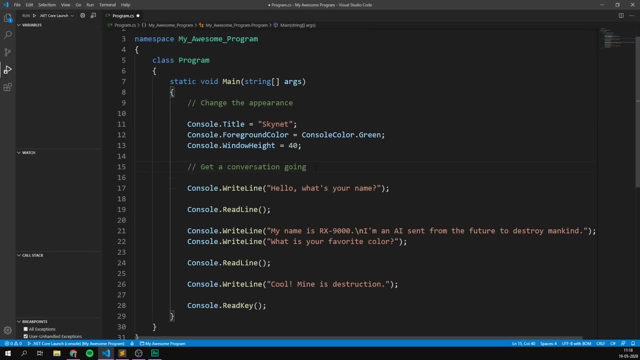 And the syntax for this is slash, slash, And here we can write a comment. So here we change the appearance of our console And then here we get a conversation going. So these comments are just for you and they won't be included when we build our program. 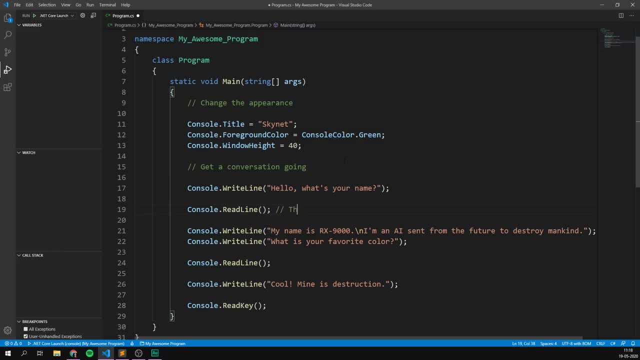 And we can actually add them after a line as well, like this. This works too Awesome. So I'm actually going to give you a challenge before you move on to the next video. The challenge is to use consolewriteLine and consolereadLine, like we just learned. 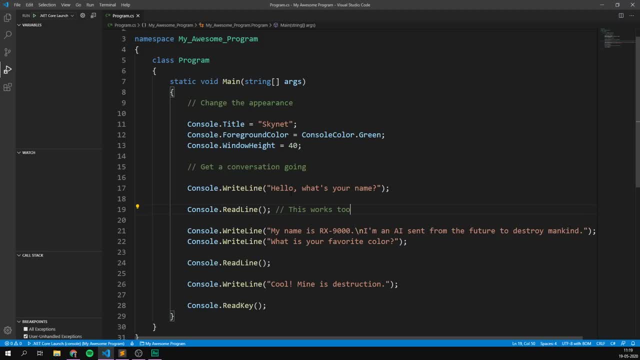 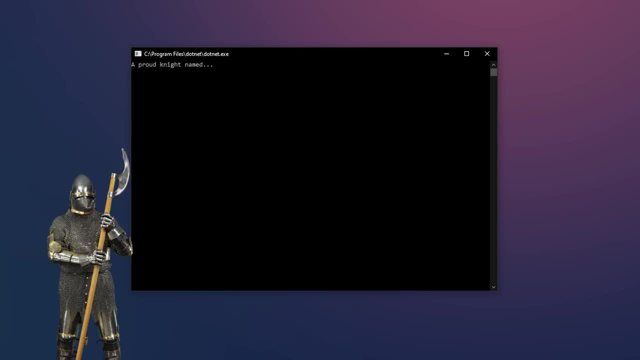 to create a short story where the user gets to determine parts of the story. Now let me give you an example. So here's one. I created a proud knight named- let's input- Eric walked into a bar. At the counter he met a- I'm going to write- talking bear. 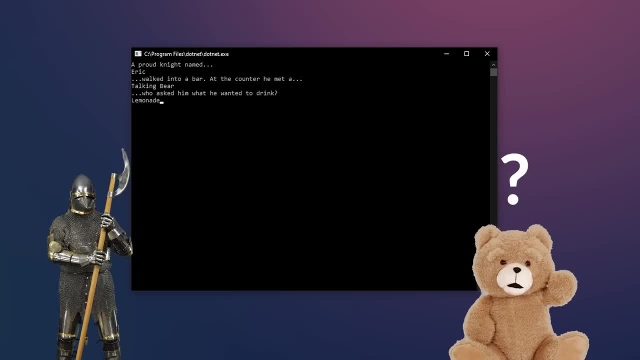 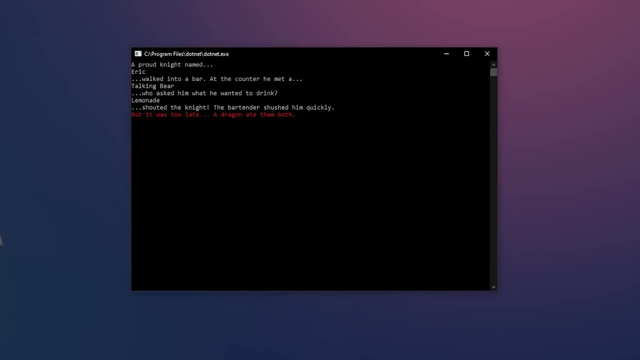 who asked him what he wanted to drink. Let's input lemonade. Lemonade, shouted the knight. The bartender shushed him quickly, but it was too late. A dragon ate them both. All right, so it's maybe not the best story ever written. 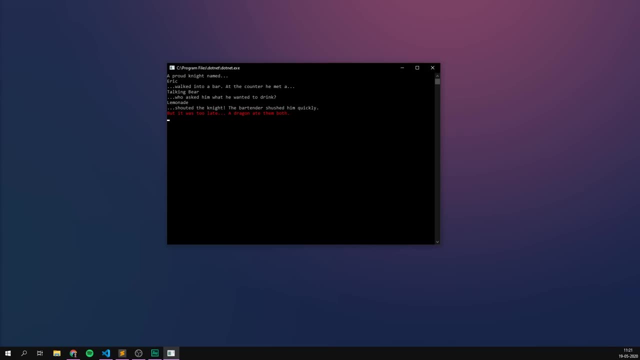 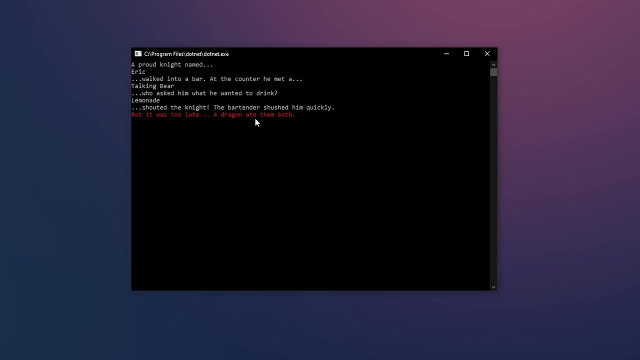 but it's still fun, because the user got to tell part of that story. And all of this is made just using consolewriteLine And consolereadLine. Notice how, at the last line here, I'm changing the foreground color. You can do this during your program. 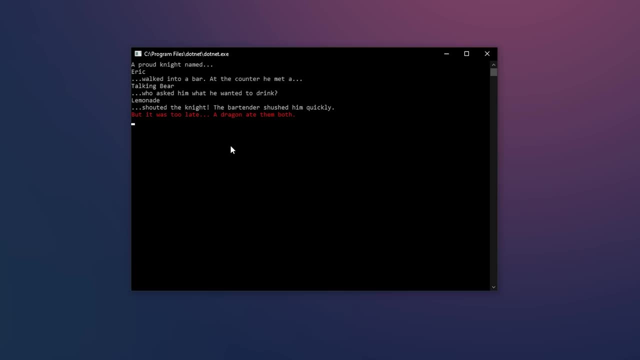 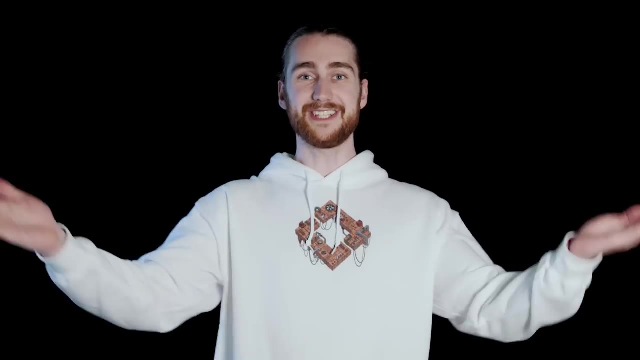 to get different line colors If you want, play around with that yourself. So that's your challenge. That's pretty much it for this video, except I have one more exciting thing to show you, which is that we completely remade the Brackeys forum. 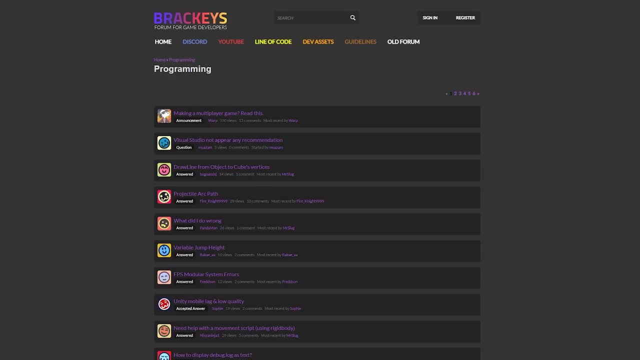 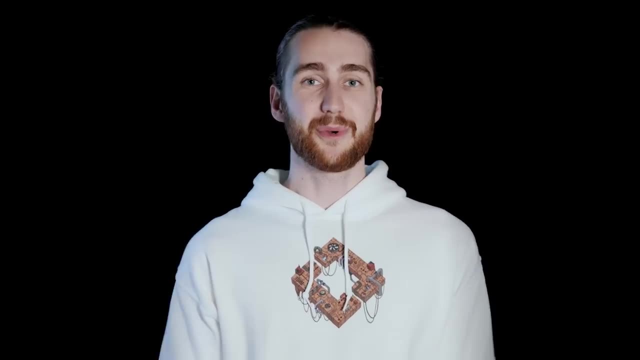 This makes it easier than ever to go ask questions, whether you are stuck or there's just something you really want to know. Simply visit forumbrackeyscom to get answers and meet fellow developers. I will also be posting the answers to the challenges. 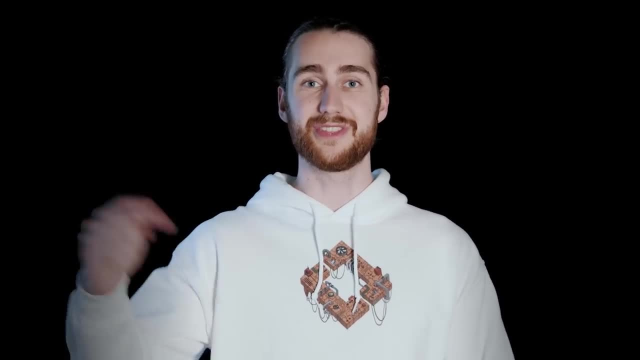 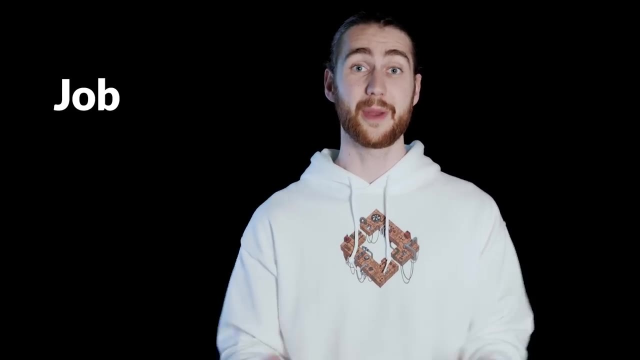 of each video on the forum. There's already a link in the description for this one. Also just want to say a huge thank you to the awesome Discord staff who created this new site and a special thanks to Job and Codemist for all the hard work.